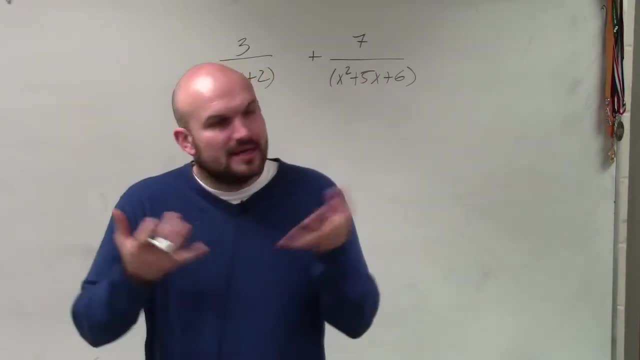 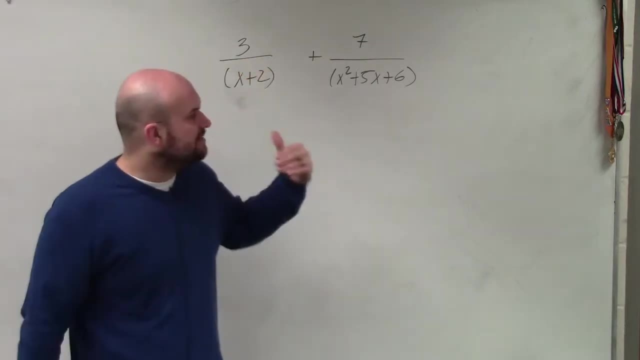 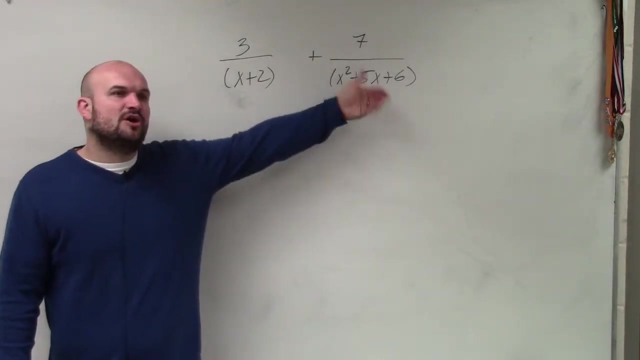 we're trying to combine this into one expression. Now, to combine this into one expression, you have to have common denominators. So the first thing we always did was determine the common denominator. However, if you guys look at a problem like this, the easiest thing to do is multiply your denominators to find a common denominator. 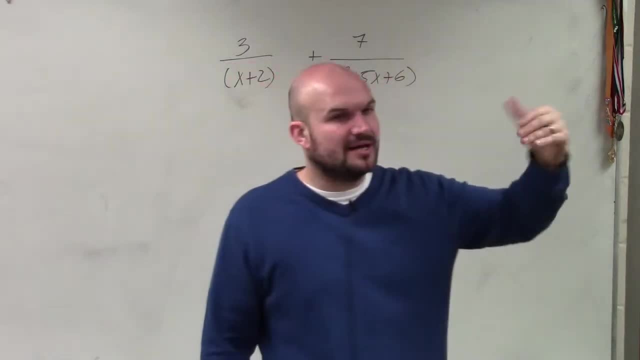 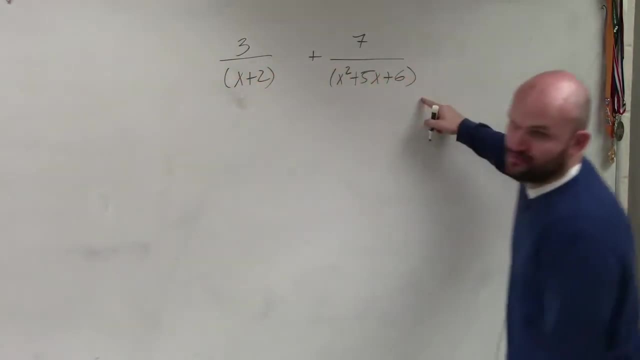 However, any time an opportunity comes for you guys to simplify, I would highly recommend factoring to have this simplified. So if I factor this right now, if I factor this trinomial, because that's the only thing I see that can be factored- 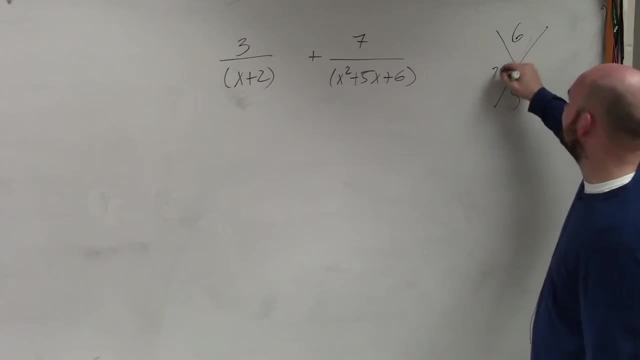 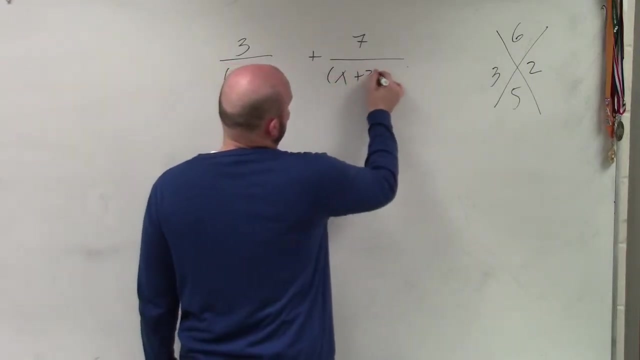 I see that's 6 and 5. What two numbers multiply to give you 6, add to give you 5? 3 and 2.. So therefore, I can rewrite this As x plus 3 times x plus 2.. 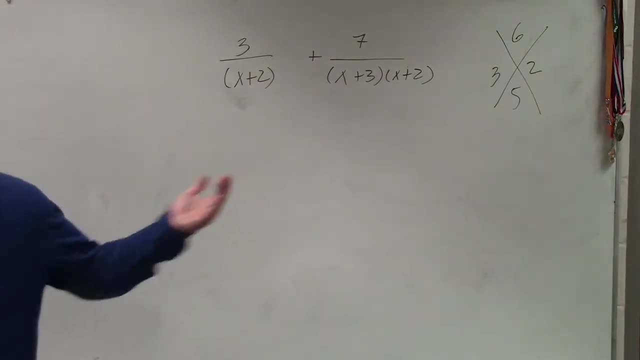 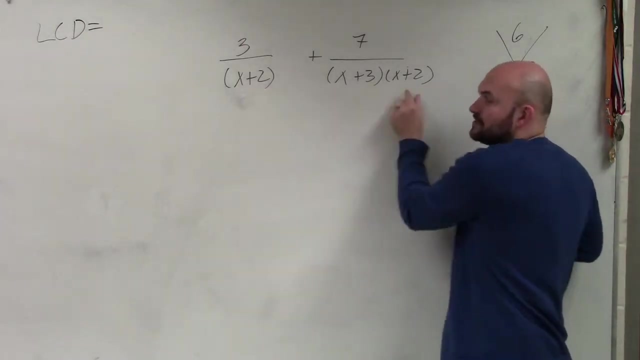 Now, what that does to help me out is now, when I'm combining them, I can determine that the LCD here is going to have to contain x plus 2 as well as x plus 3.. I don't need to multiply these, because x plus 2 is the same. 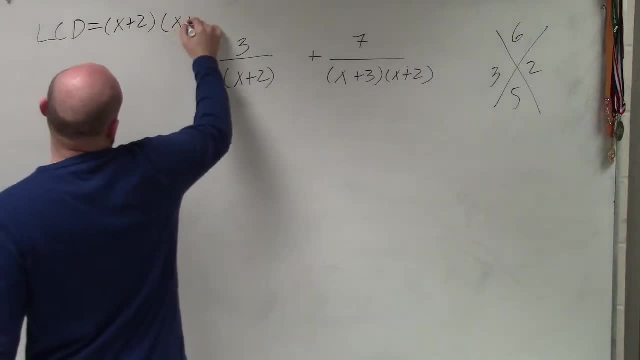 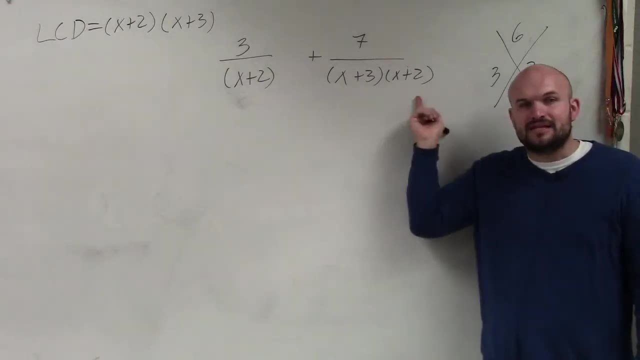 So the LCD is going to be x plus 2 times x plus 3.. So if you guys know, Notice what's by factoring I'm able to allow. this is already my LCD. All I need to do is get this to have the same denominator. 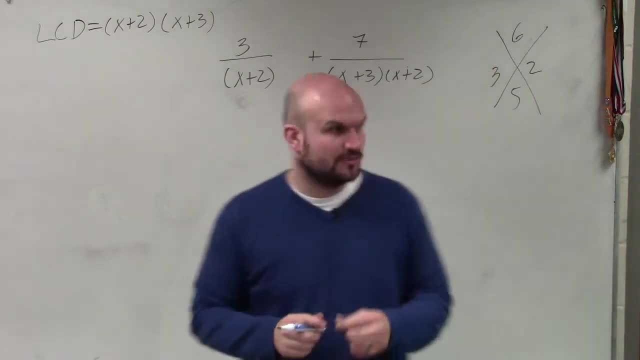 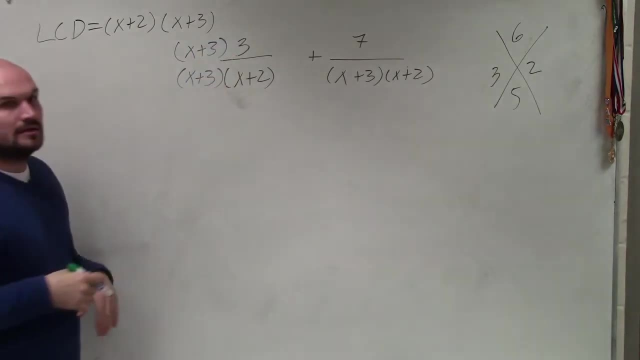 I really, really try, guys, but I'm sorry, I mean, it's really just a waste of time. So here I'm going to be multiplying by x plus 3 over x plus 3.. What that does is now: that gives me the same denominators. 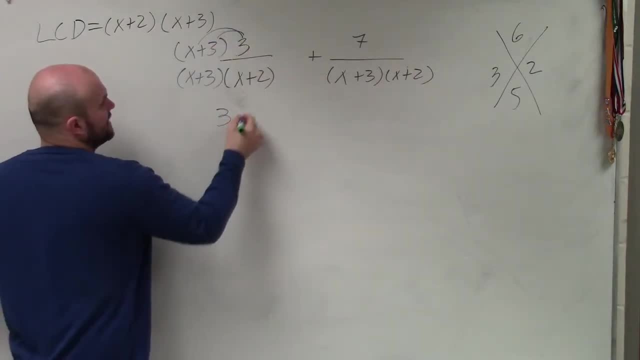 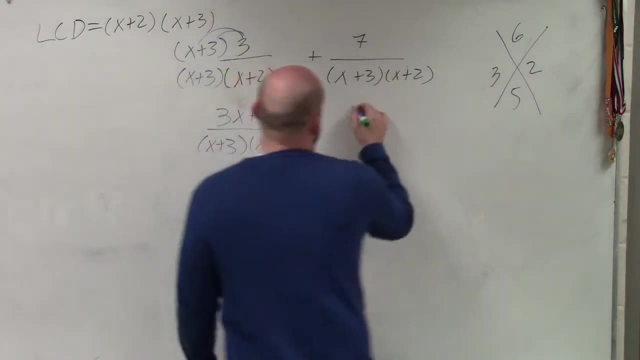 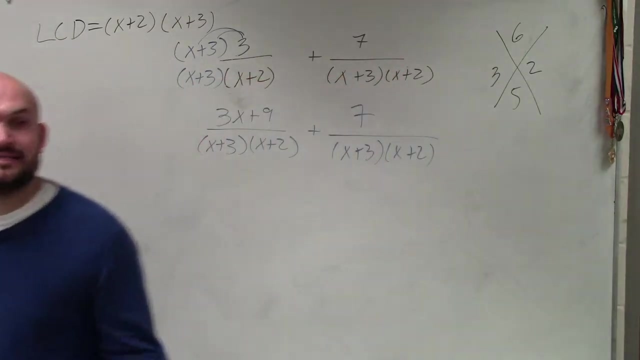 I apply distributive property. So what I obtain is 3x plus 9 divided by x plus 3 over x plus 2 plus 7 over x plus 3 times x plus 2.. Now you guys can see that my denominators are exactly the same. 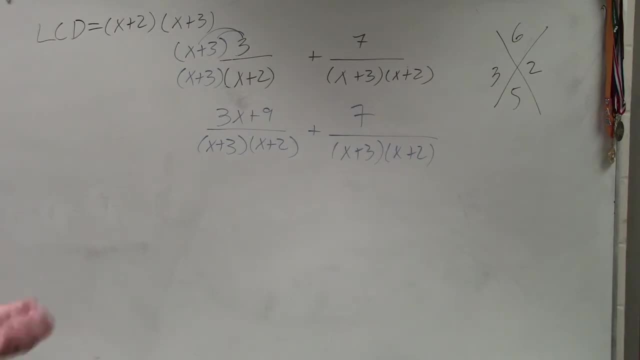 Just like if I had 1 fourth plus 3 fourths. right, You keep the denominators and add the numerators. So therefore, well, the only thing I can add is the 9 and the 7, which is 16.. 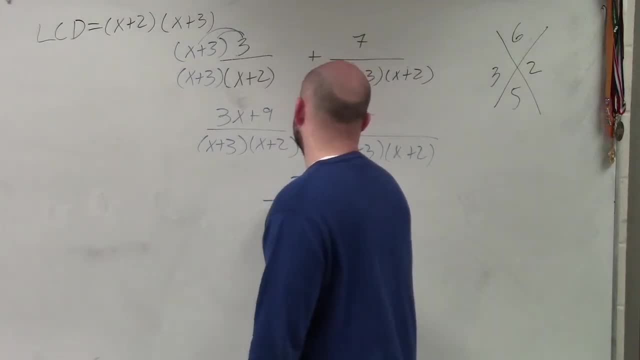 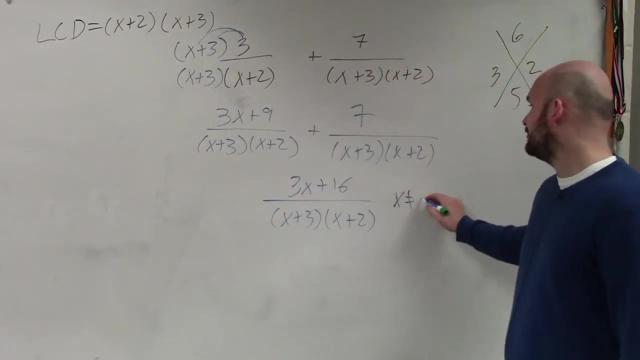 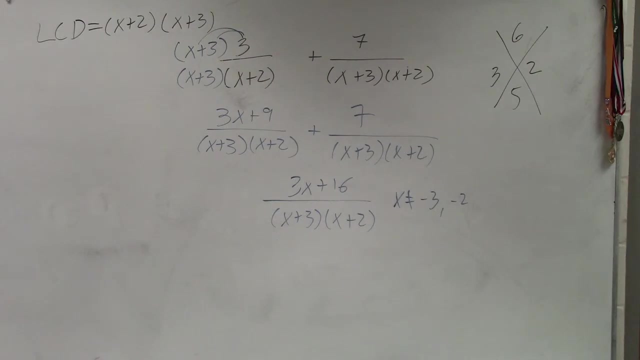 So this becomes 3x plus 16 divided by x plus 3, times x plus 2, where x cannot equal negative 3 and negative 2.. Everybody see that. See what I did. So it's really, really.